We can see that the result of ViewShot AD is very similar to the result of Ambutech AD. We can see that the result of ViewShot AD is very similar to the result of Ambutech AD. We can see that the result of ViewShot AD is very similar to the result of Ambutech AD. 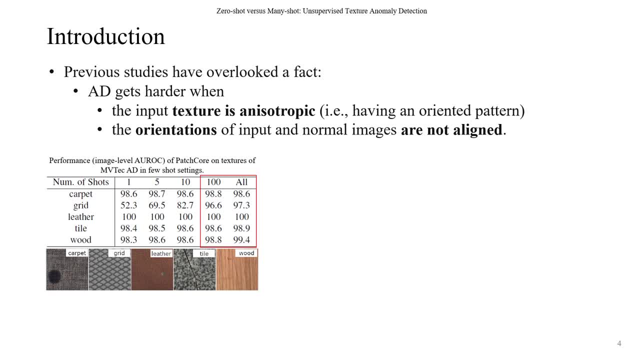 We can see that the method works well when we have many normal samples. However, when we have fewer normal samples, detection accuracy varies greatly among these textures. As compared with the case of using more than 100 samples, ViewShot accuracy deteriorates significantly for grit and modestly for wood. On the other hand, 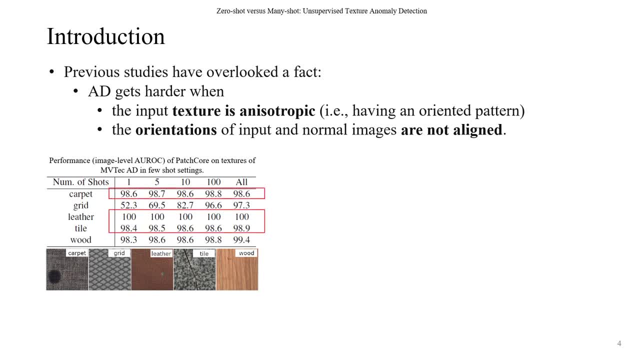 it barely decreases for carpet and tile. There is even no change for leather. What makes the difference? There are several factors leading to these differences, such as the different orientation of the texture, For instance. the most vital one is the isotropy of texture. 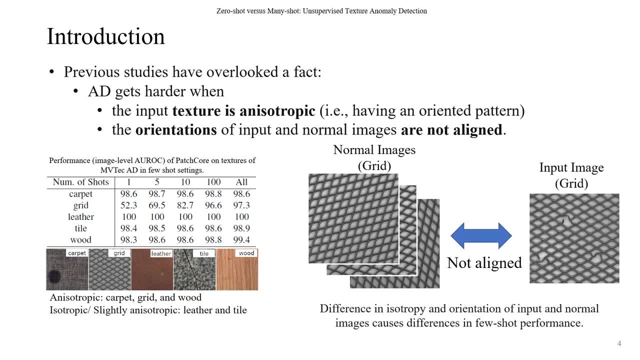 which means whether or not a texture has an orientation. For the Ambutech AD textures, carpet, grit and wood are anisotropic, whereas leather and tile are isotropic or only slightly anisotropic. The difference in isotropy causes the above difference in ViewShot performance, Because if the input image has a different orientation with normal samples, as shown here, it becomes hard to distinguish normal and isotropic. 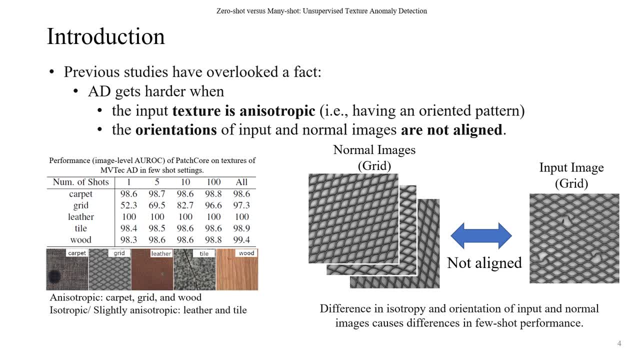 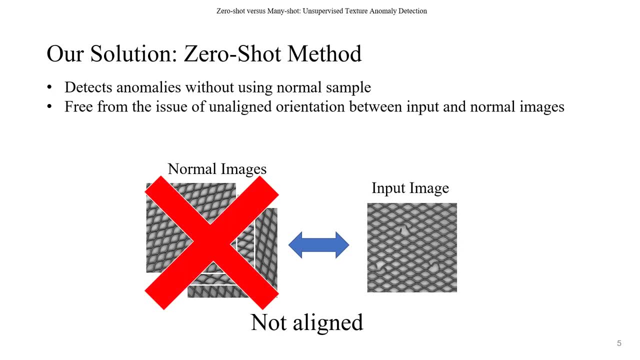 Anomalous region. The more normal samples we have, the more likely we have a particular normal sample having an aligned orientation with the input image. We propose a zero-shot method. This method detects anomalies without using normal samples. Therefore, it is free from the issue of unaligned orientation between input and normal images. 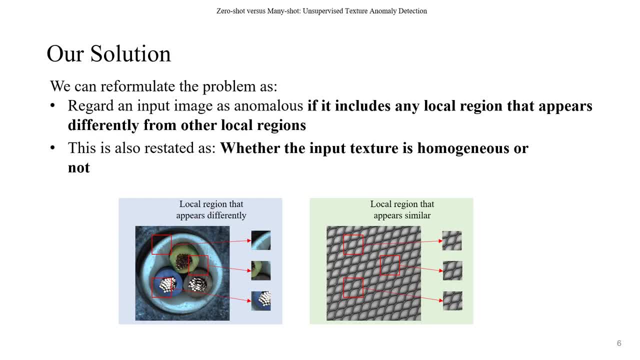 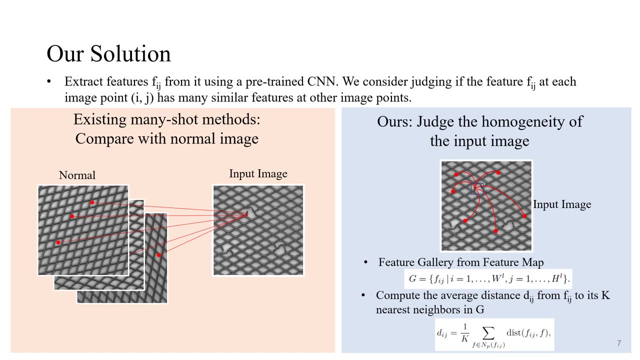 We can reformulate the problem as we regard an input image as anomalous if it includes any local region that appears differently from other local regions. This is also restated as, whether the input texture is homogeneous or not, We extract input image features to create a feature: negative G. 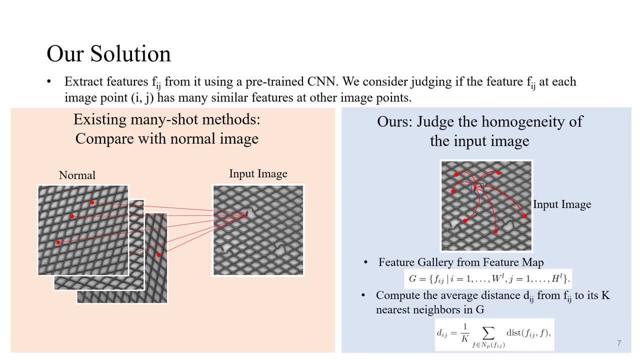 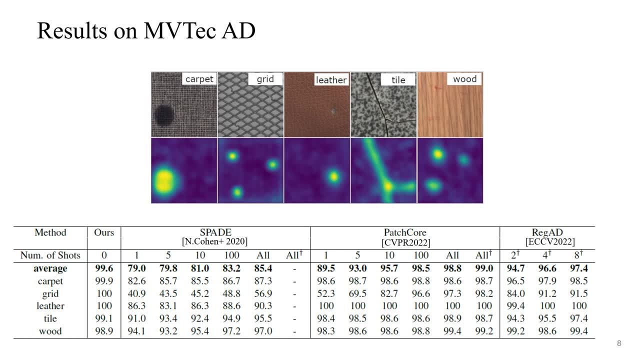 and compute the distance between G and features at each image point to judge the homogeneity of the image. Thisusi got our título de alguna parte. This subtitle is for wollte Please sit in our poster session for more details- 7-0.. First we show the performance of our method on 5 textures of Ambutech AD. 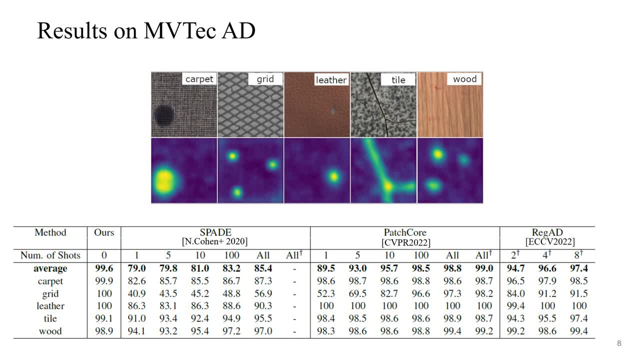 Our method outperforms paed and patchcore even with 100 normal images. Our method outperforms paed and patchcore even with 100 normal images. compensates for the orientation misalignment issue, but it may not be perfect. Our method is free of this misalignment issue. For further verification, we test our method on a dataset.